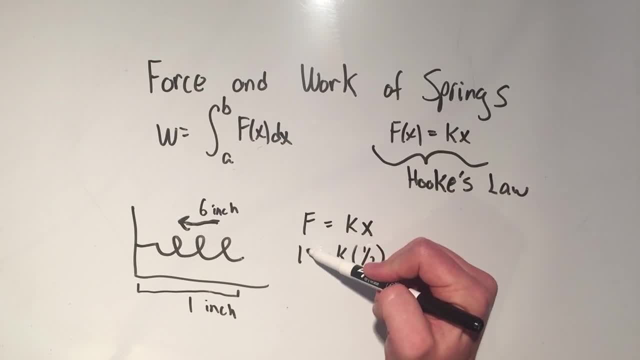 it in, but it doesn't really matter. I said that the force required to do that was 10, which means I can solve for my k, I can solve for my spring constant by multiplying by two and I'm getting that my k is 10.. So I'm going to do that, And I'm going to do that, And I'm going to do that, And 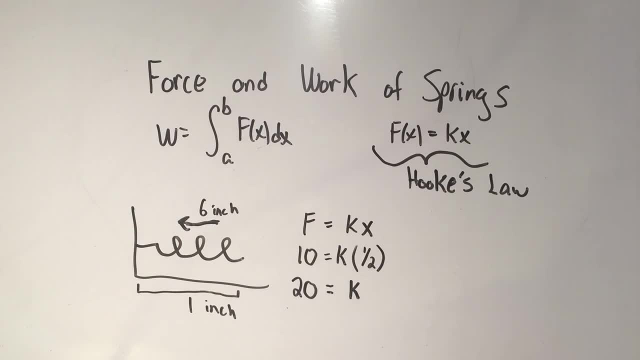 it's going to be 20.. So that information, if they give you a problem on this, they'll have to give you. they'll have to either give you the spring constant or they'll have to tell you it took so much force to push it or pull it this much. And once you have k you can answer other questions. 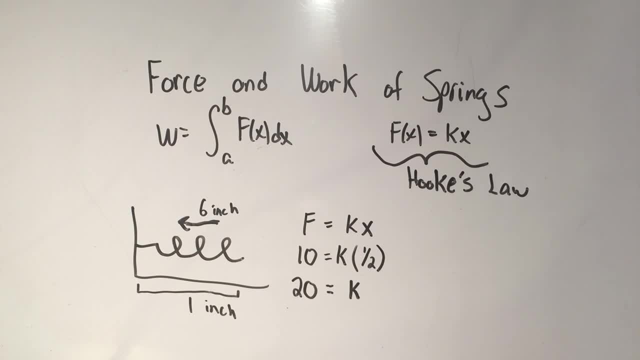 So let's just say I wanted to know how much work it would be if I took this string and I stretched it out one inch more. So if you can imagine me taking this string, spring and pulling it out till it was a whole out- another inch, that makes sense. 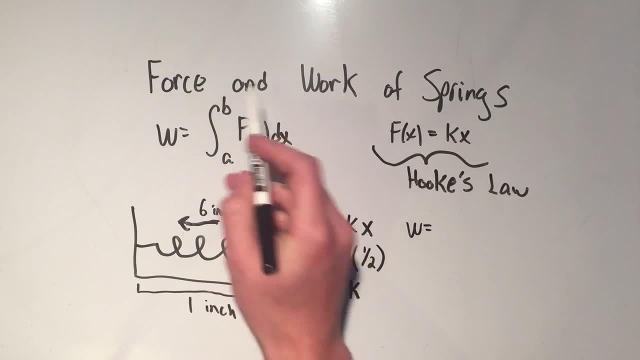 well, I'm just gonna do this formula right here. so if I'm have it as natural position and I stretch it one inch, that'll be the definite integral from 0 to 1, and then I need to integrate the force function, which is K times X. I. 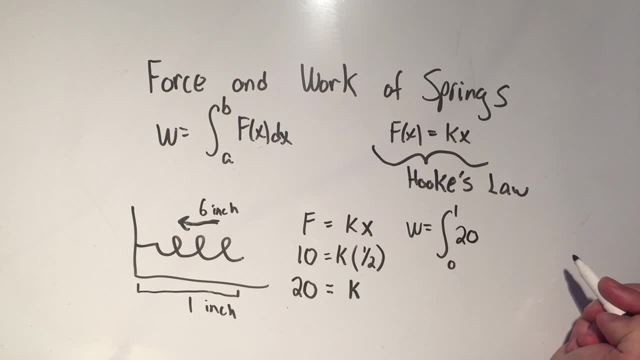 just found K. K was 20 and then I put an X here and then I just need DX, and now this is a very easy definite integral to solve. so we can just solve that by adding 1 to the power, dividing by the new power and evaluating from 0 to 1- 20. 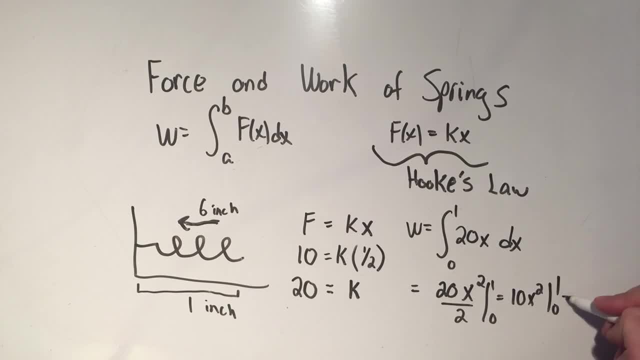 over 2 is 10, and if I plug in 1, 1 squared, if I plug in 0, that's 0 squared. 0 times anything is 0. 1 times 1 is 1. so the amount of work to do this would be 10. so there is your introduction to springs and doing work. 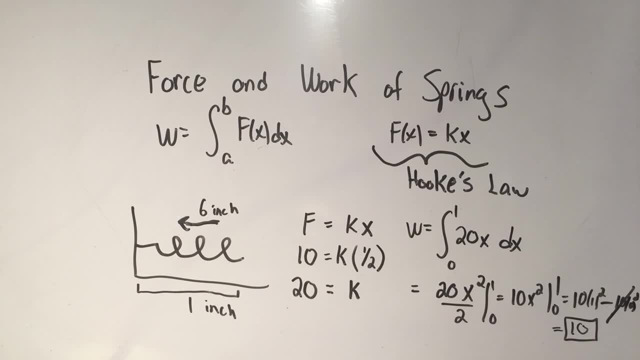 it's really just the same formula as work with definite integrals. you just have to remember Hooke's law over here that the force of a spring is K times X. hope you got something out of it. thank you very much for watching and have a great day.